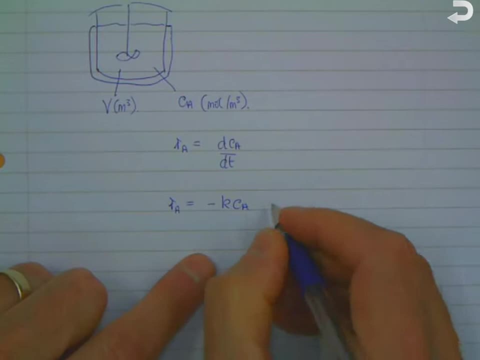 got first order reaction in our starting component A and we've got K as the kinetic rate constant, The first order rate constant because it's first order. it has units of the first order Seconds to the minus one. This is negative because the reaction rate is negative, because 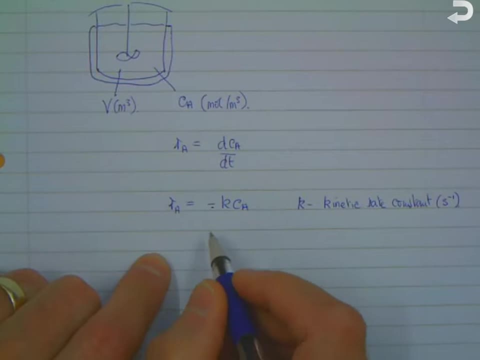 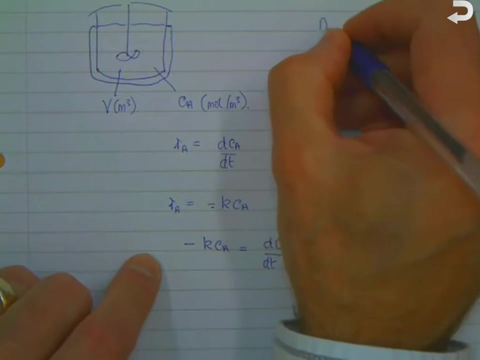 Ra is the starting material which is being consumed. So we've got Ra equals minus K times KCa. If we substitute that into that and combine the two equations, we get that minus K times Ca is equal to dCa. Now I've got to make a further assumption in order to integrate that expression And 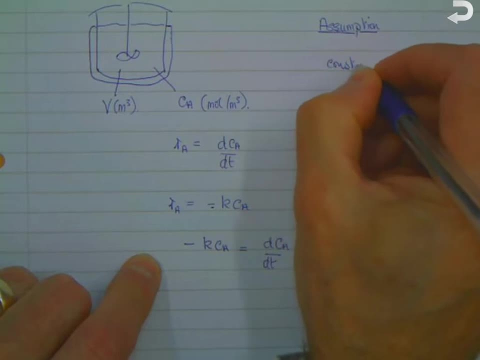 that is, that we've got constant temperature, or at least that the temperature is close enough to constant. So we've got constant temperature, Or at least that the temperature is close enough to constant, Or at least that our value of K can be assumed to be a constant. 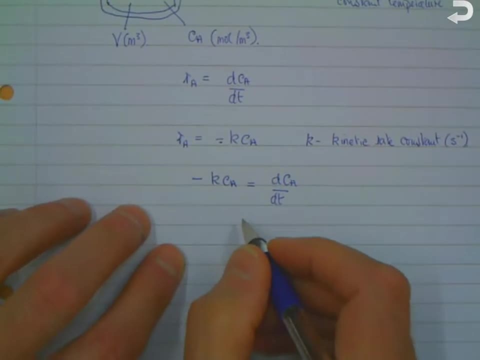 And so if K is constant, then we can integrate this expression And we get minus K times integral dT And call it integral dCa over Ca And I've got to have some limits on these. So I've got to have some limits on these And you'll see I'm integral ca over ca. 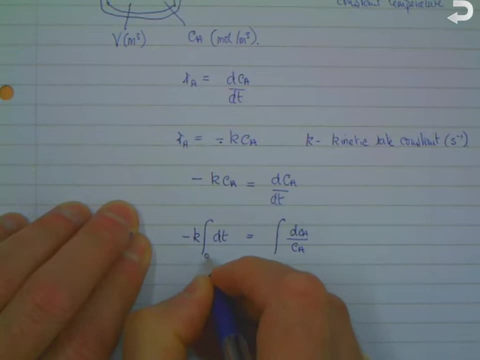 limits on these integrations. so we're going to integrate from time t equals naught. at which point? so that's the starting point of our reaction. so we're going to assume that we've got a starting concentration of our component A, of C, A naught. that's, at times t equals naught and then at some time t the. 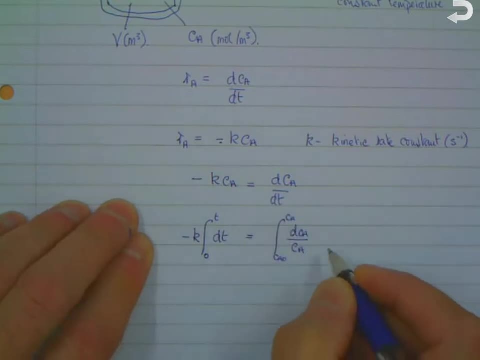 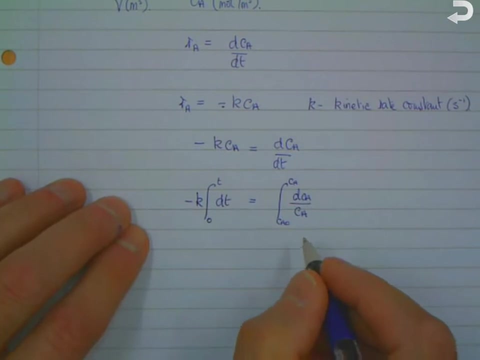 concentration of A has gone down to a new value, C, A, so we can integrate that. we get that. that's an easy integration. so k is constant because of that assumption we've made and you've got, minus kt, between limits of 0 and t, an integral of 1 over C, A, d, theta. 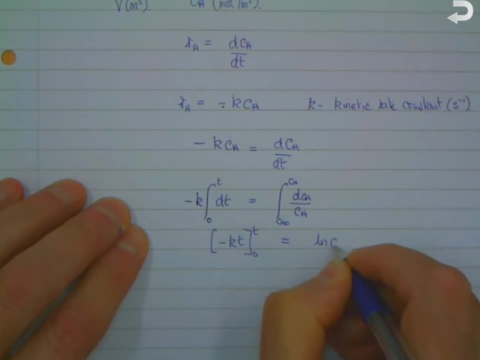 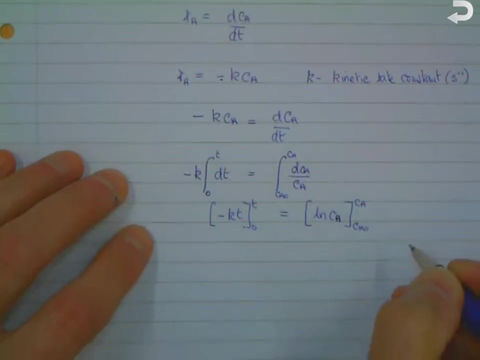 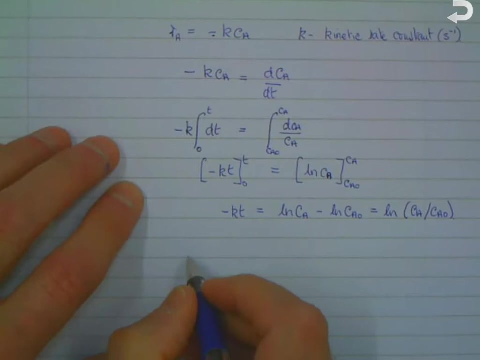 is log term, log of C A, and again that's between those limits of C A, C A naught and C A and that gives you minus kt equals log C A, minus log C A naught, which is simply log of C A divided by C A naught. and if you want to, 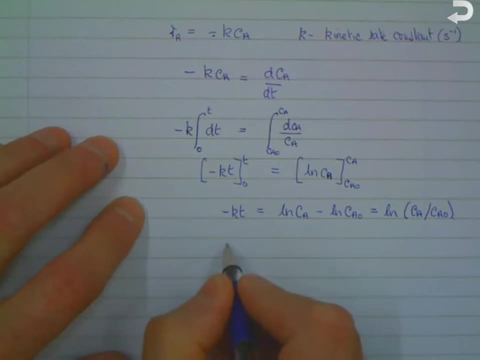 calculate the required time for a given final concentration. so your your battery action time to achieve a final concentration of c-a and the final concentration of c-a. Then you could just rearrange that slightly. Take minus k over to that side, divide both sides by minus k. You get that equals t, equals minus 1 over k times log cA over cA naught. 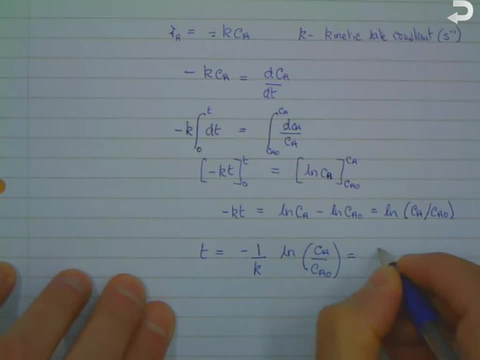 And it might be quite convenient just to get rid of that minus sign That gives you 1 over k. So if you take that minus sign in there you can invert the log That gives you cA naught over cA. So that's an expression for the required reaction time to achieve a final. 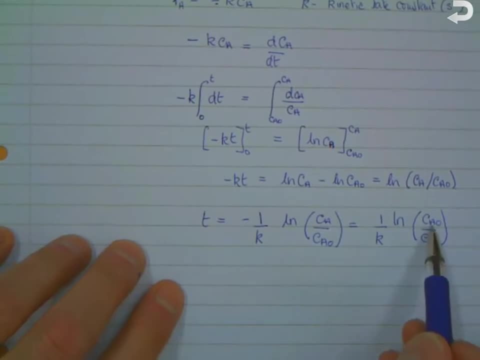 concentration of cA from an initial concentration, cA naught. if you've got a first order kinetic rate constant, You can go back up here though, and you could raise, take the exponential of both sides of that equation in order to get rid of the log, And that gives you exponential.